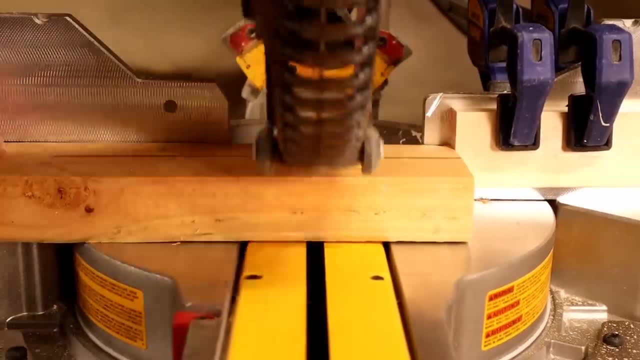 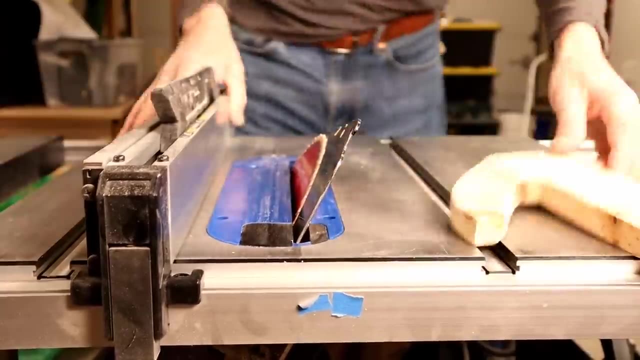 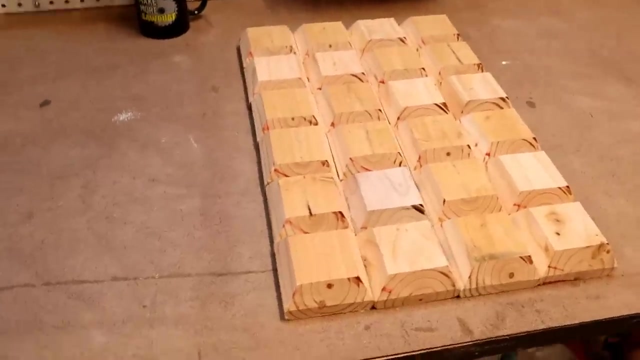 The idea of these small cost, high profit videos is to get you to think about what you can do with any scrap wood laying around. Once all of the blocks are cut, I set my table saw to 30 degrees and the fence to 3 inches. Then I run each block through on all sides With the angle cuts on all. 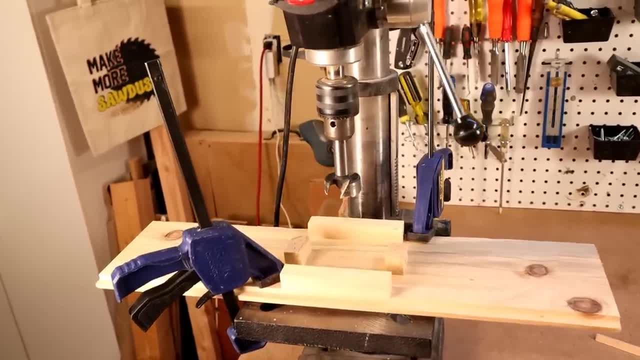 the blocks complete, it's time to go to the drill press. Now I set up a jig that allows me to keep each block in place and centered. I'm going to set up a jig that allows me to keep each block in place and centered. Now I set up a jig that allows me to keep each block in place and centered. I'm 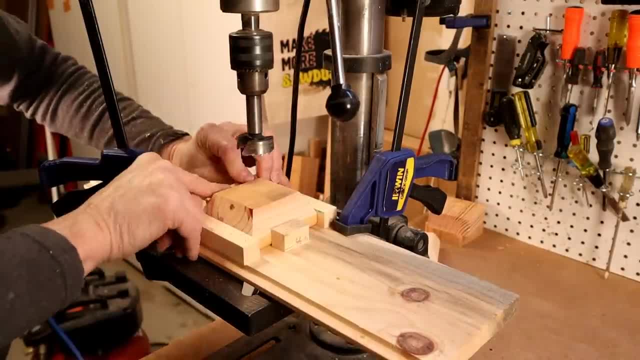 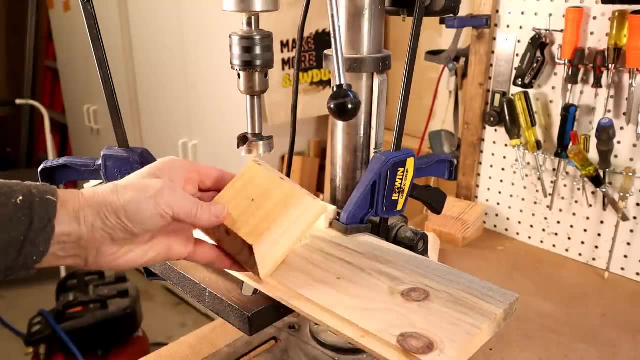 going to set up a jig that allows me to keep each block in place and centered While I use a one and a half inch forstner bit to drill about a third of the way down. It took a bit of adjusting and re-clamping to get to the point where I was satisfied with the alignment. Now it's just a. 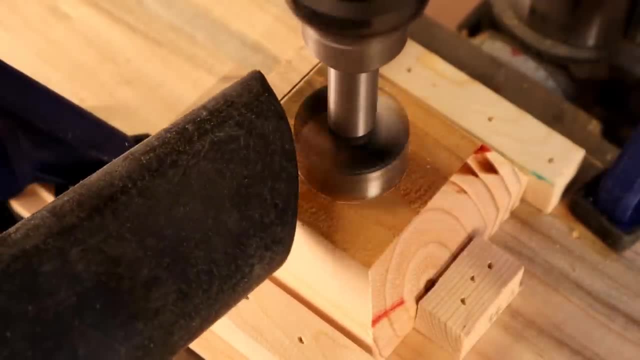 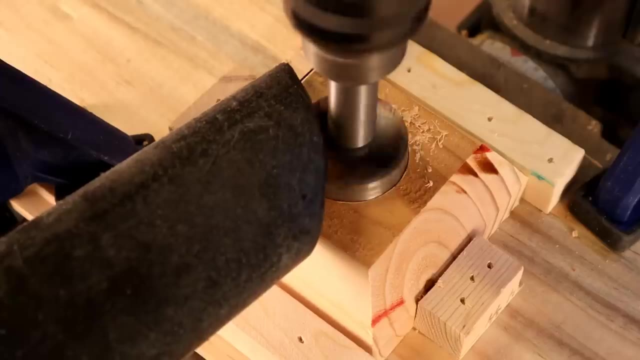 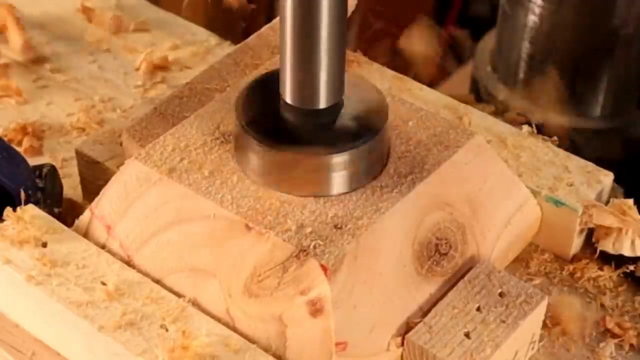 matter of placing the block and slowly lowering the drill bit. You can see I have my shop vac nozzle in the other hand, close by. Let me show you what happens. if you don't do that. You can imagine the amount of shavings I'd have to clean up after drilling 24 blocks. 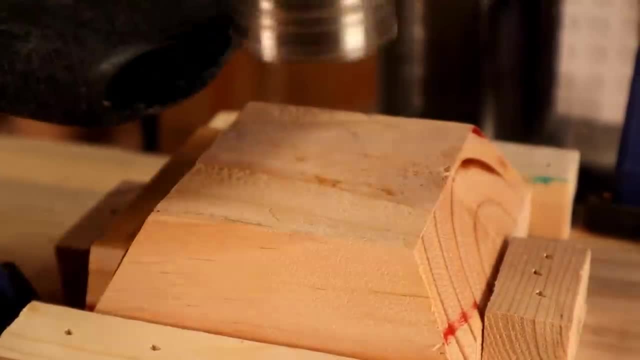 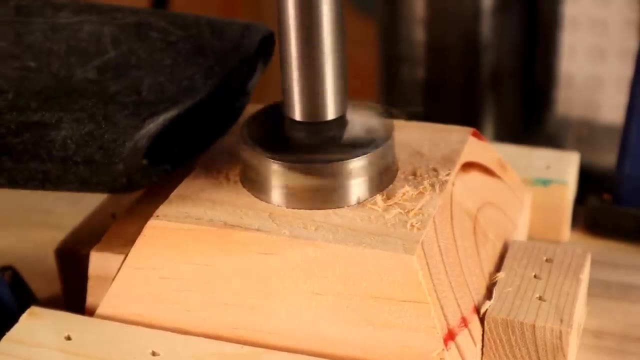 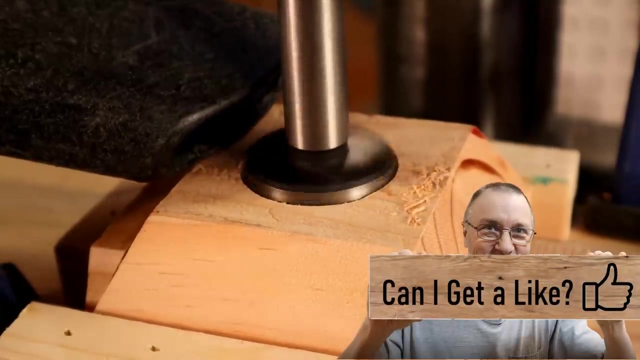 No, thank you. So do you have an idea what this project is? yet Tell you what? pause the video. write your guess in the comments before the big reveal. Maybe it's just me, but watching this video footage of drilling a hole in this block is somehow satisfying to me. You know work. 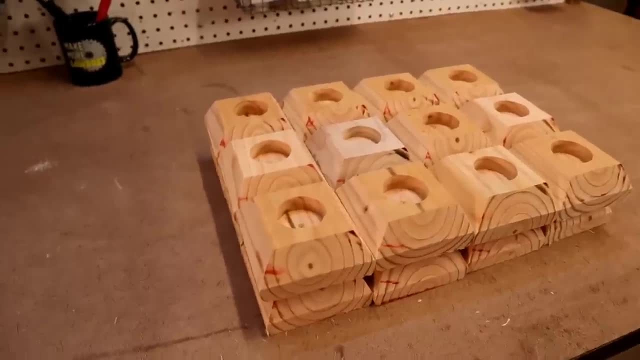 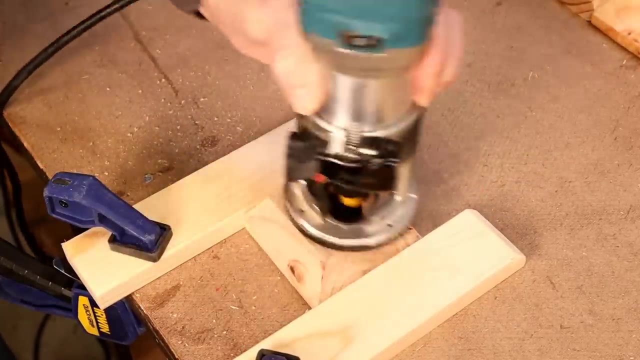 is getting accomplished in a somewhat clean and efficient way and the creation is coming to life. My next step is to round over the sharp edge of each hole with my palm router. I'm using an eighth inch bit Now. I started out by holding a block. 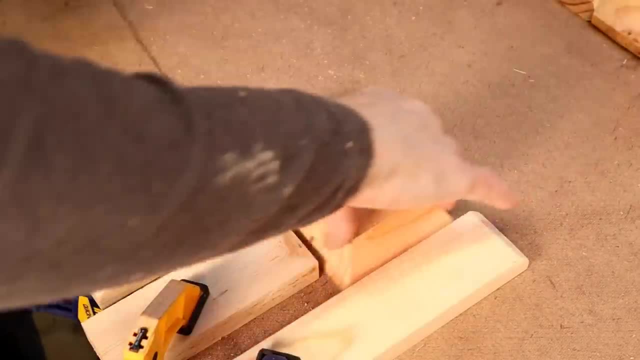 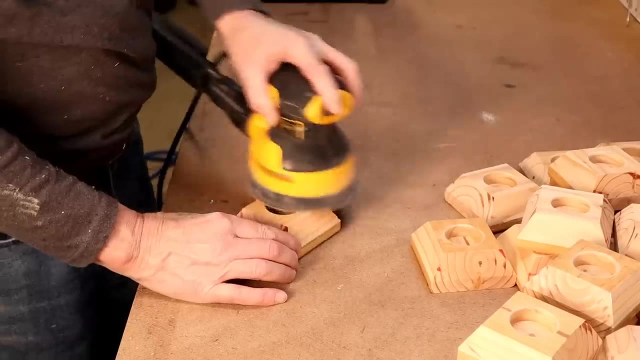 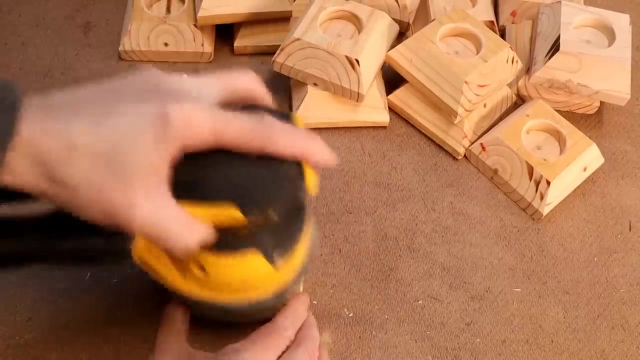 but really wasn't comfortable having my hand that close to the router, so I did some improvising along the way. If you're gonna do this, just use caution and be safe. Now the part I really don't enjoy: Sanding, and sanding and more sanding. 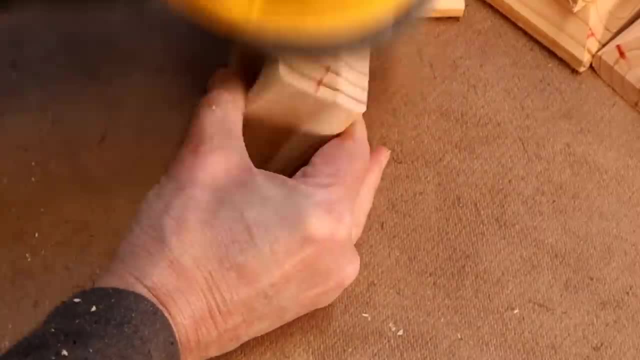 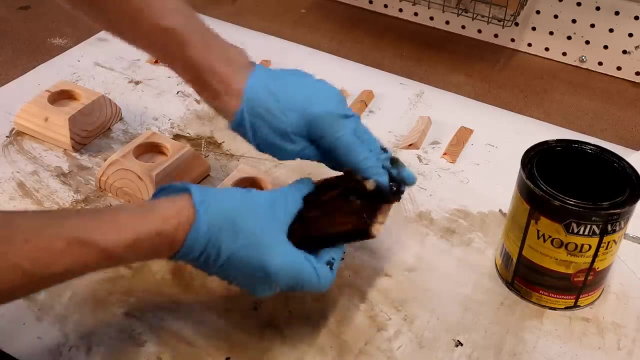 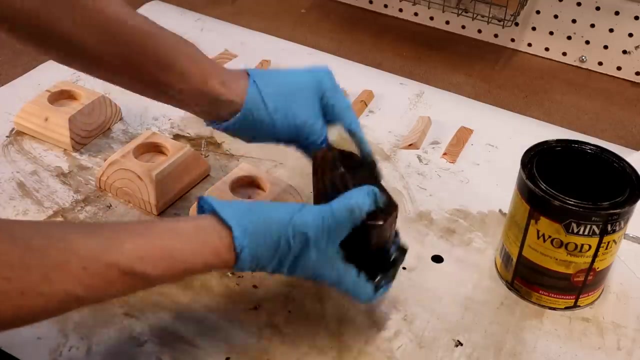 You know, it's not so bad watching the video footage back, but creating it not my favorite part. Okay, some stain. I'm just gonna do four blocks here. I haven't decided yet what the other colors I want to use are going to be, but I'll show you now the screenshots of this item for sale before.